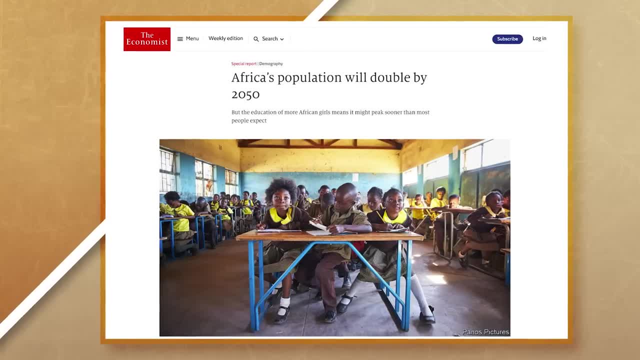 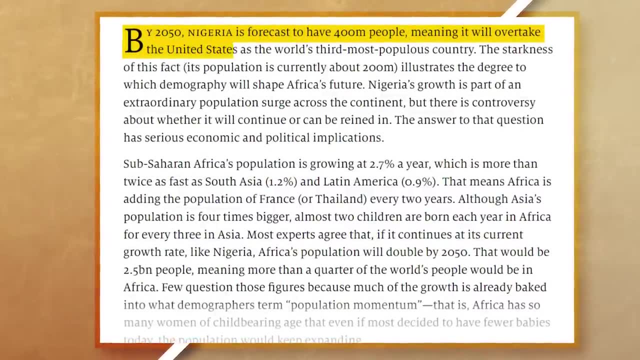 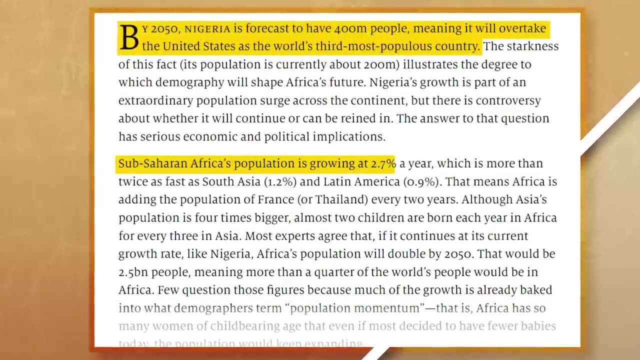 in the world that are experiencing a population boom. According to The Economist, by 2050, Nigeria is forecasted to have 400 million people, meaning it will overtake the United States as the world's third most populous country. And, as of today, Sub-Saharan Africa's population is growing at 2.7% a year, which is more than 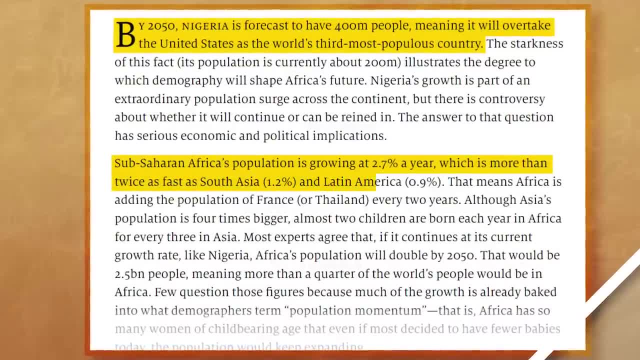 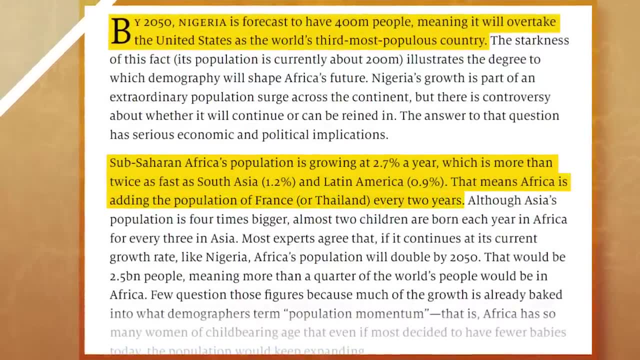 twice as fast as South Asia, which is at 1.2%, and Latin America, which is at 0.9%. That means Africa is adding the population of France or Thailand every two years. So which is it? Is the global population crashing or is it exploding? 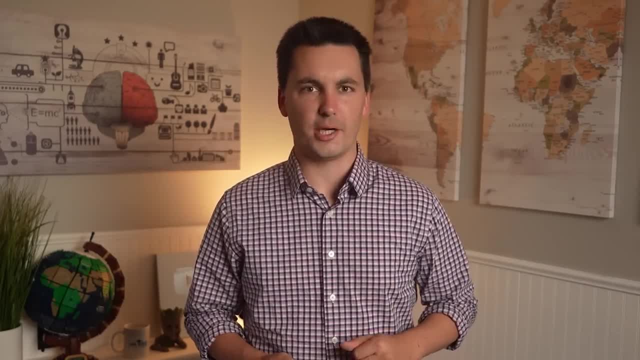 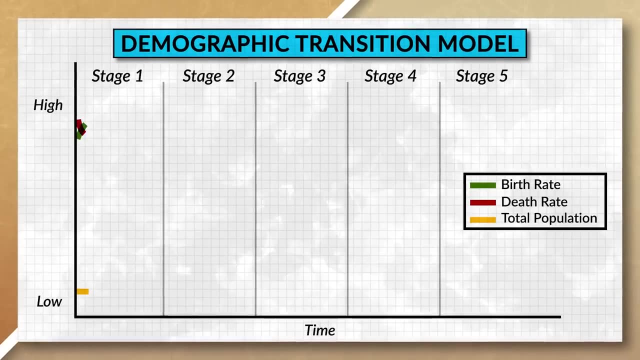 To answer this question, we have to understand the demographic transition model. It's a model that has five different stages and it focuses on different economic and social developments of a society. In the first stage, societies have a high CBR and CDR, which actually end up creating 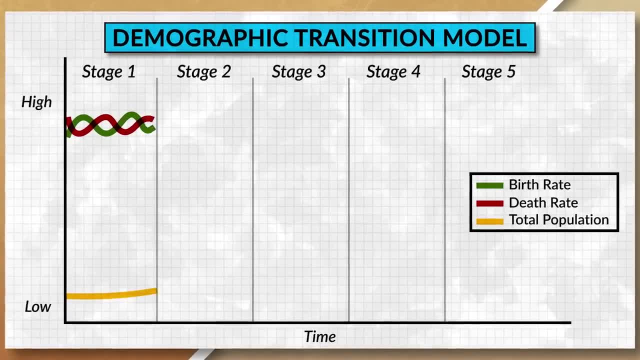 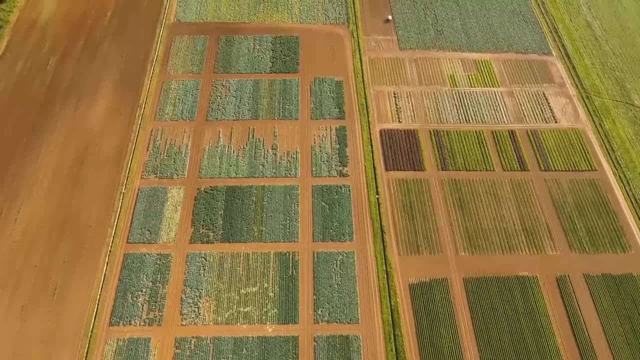 a low NIR, since the births and deaths end up canceling each other out. Societies in this stage are traditionally lacking sanitation, medicine, contraceptives and have more of an agricultural-based society. The majority of people work in subsistence agriculture, which is when people produce. 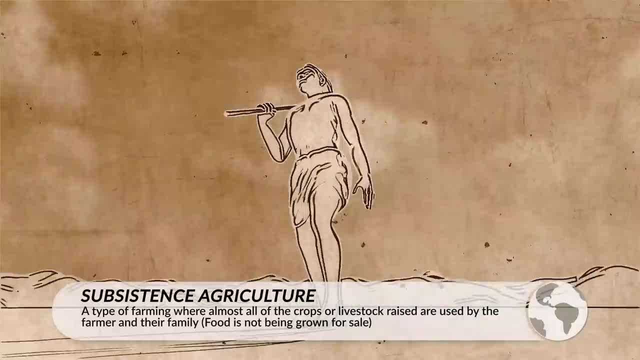 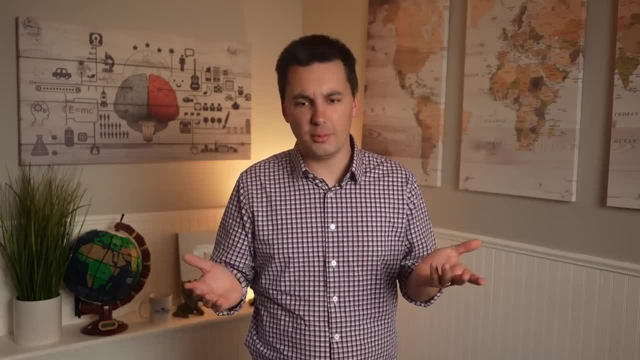 food for themselves and not for sale. We can see that during this stage, migration is often focused around the search for food. Here, people are just trying to meet their basic needs. In fact, the majority of human history actually took place during this stage. 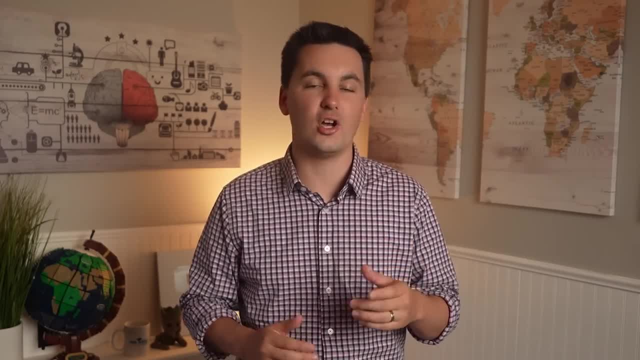 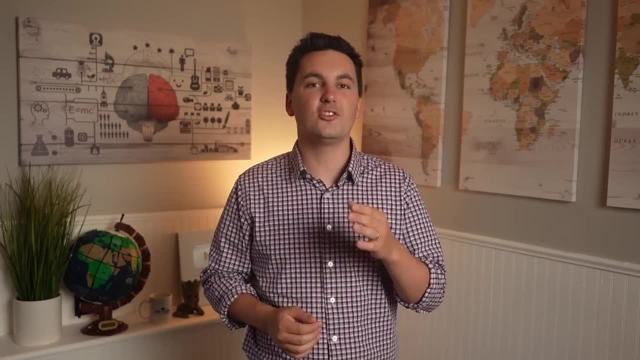 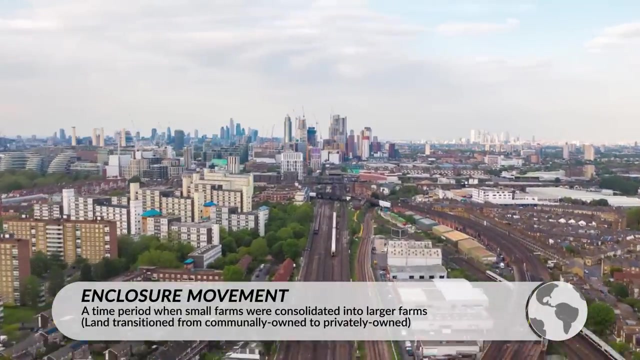 But as of today, there are no longer any countries that are in this stage of the demographic transition model. Now, once the Industrial Revolution happened, we started to see countries and societies transition into stage two of the demographic transition model. The Industrial Revolution led to the enclosure movement, increased rates of urbanization. 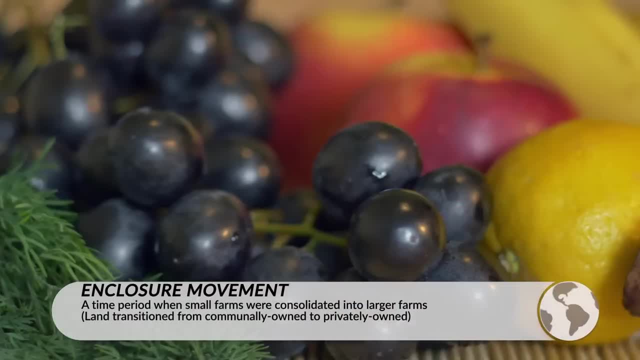 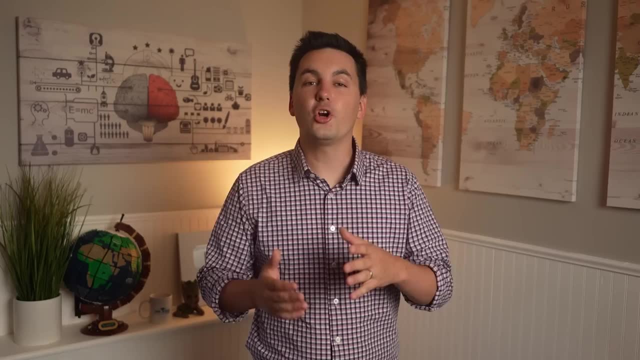 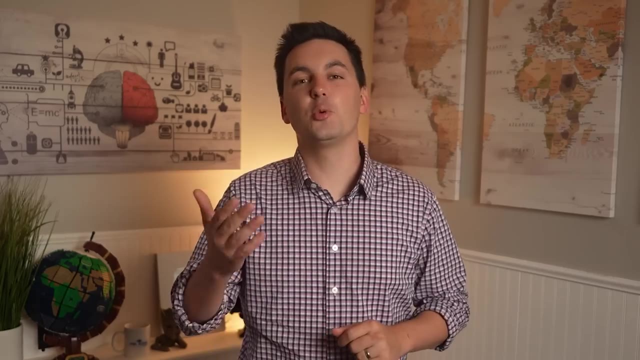 allowed for more specialization in society, increased society's food surplus and allowed for advancements to be made in medicine, which would eventually lead to the medical revolution. Europe and North America were one of the first regions to enter stage two, due to the diffusion of the Industrial Revolution. 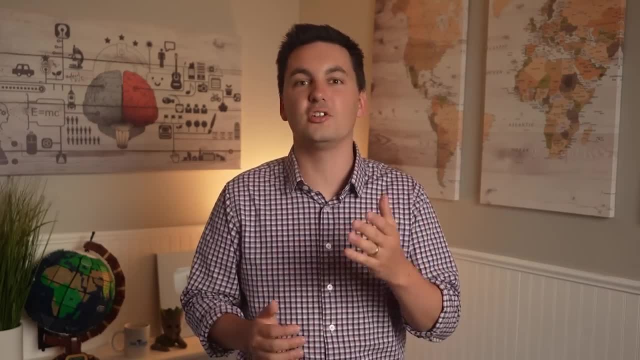 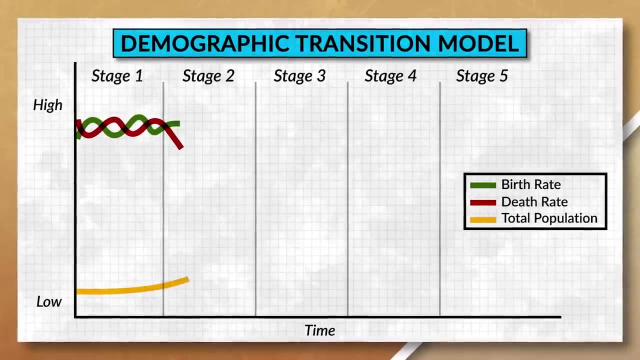 Eventually, we saw Africa, Asia and Latin America start to transition into stage two thanks to further diffusion of technology And due to this transition, we saw the industrial revolution become a major part of the global population. Countries in stage two continue to have a high CBR, but they start to see their CDR. 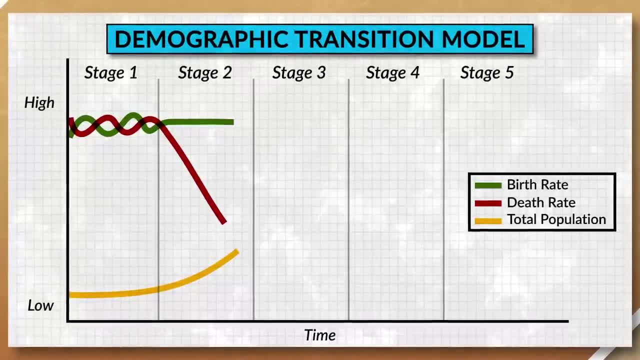 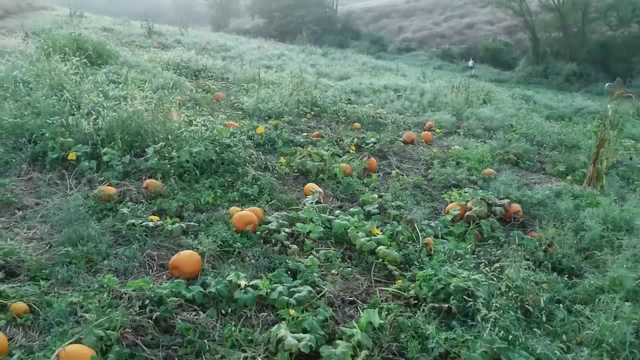 decrease, which leads to a population boom, as the CBR and CDR no longer cancel each other out. During this stage, societies increase their knowledge in medicine, improve their agricultural production, increase their food surplus and lower their IMR and CDR, all of which leads 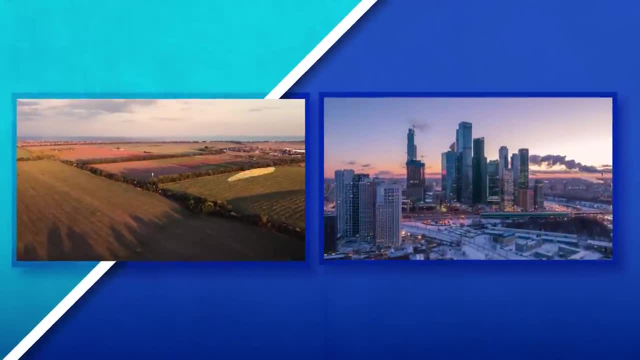 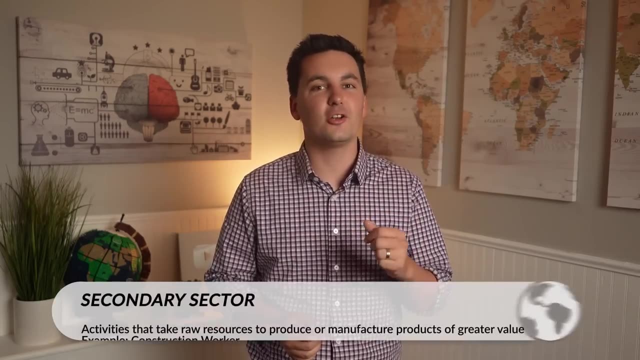 to a population boom. During this stage we also start to see increased rates of migration to urban areas. This is due to economic opportunities in the city, in the secondary sector of the economy, and also due to the fact that many of the subsistence agricultural production is now 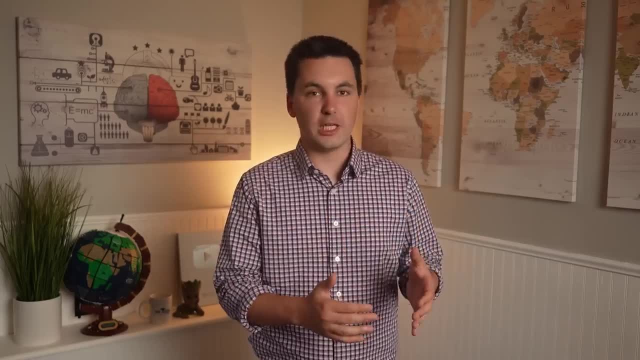 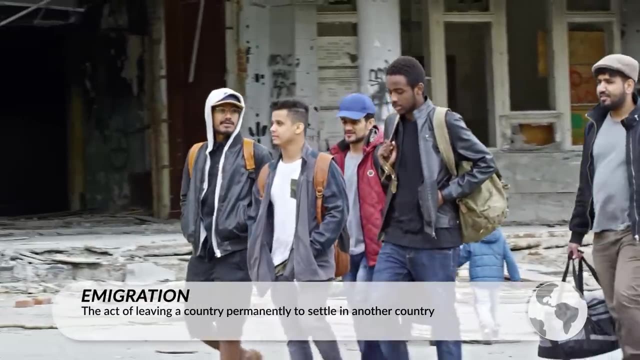 shifting over into commercial agriculture. Besides people moving from rural areas to urban areas, we may also see increased emigration, as more migrants will seek economic opportunities in core countries or more developed countries. Today, we can see that countries like Afghanistan are in stage two of the demographic transition. 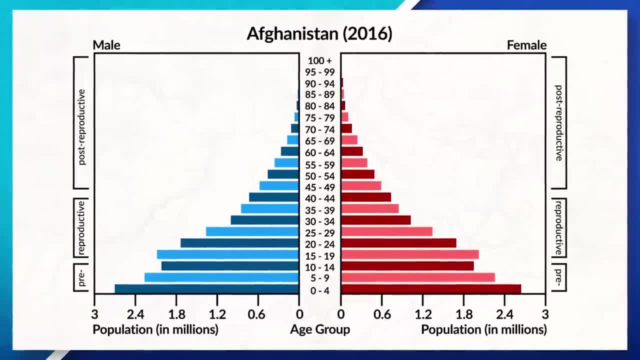 model, as seen here in their population pyramid. As you can see, the majority of Afghanistan's population is in the pre-COVID era. This means that the majority of the population is in the pre-COVID era. This means that the majority of the population is in the pre-COVID era. 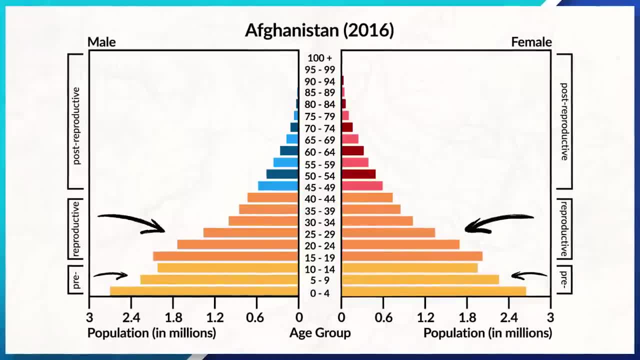 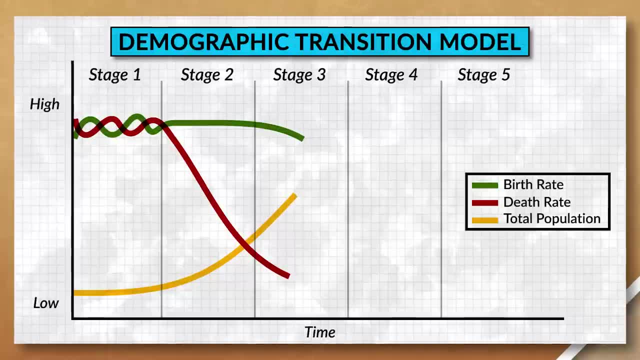 This means that the majority of the population is in the pre-reproductive years and reproductive years, which shows that the country has an expanding population. Eventually, countries start to move into stage three. During this stage, the CBR starts to decrease, along with the CDR continuing to decrease. 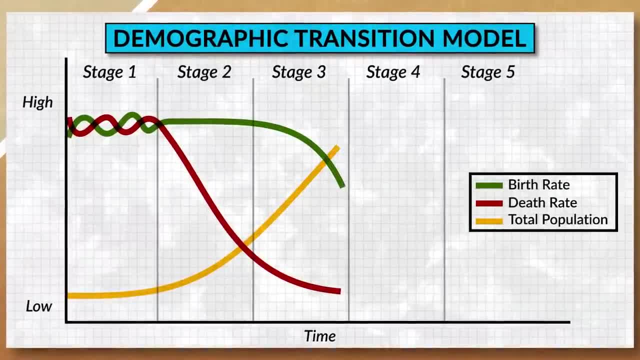 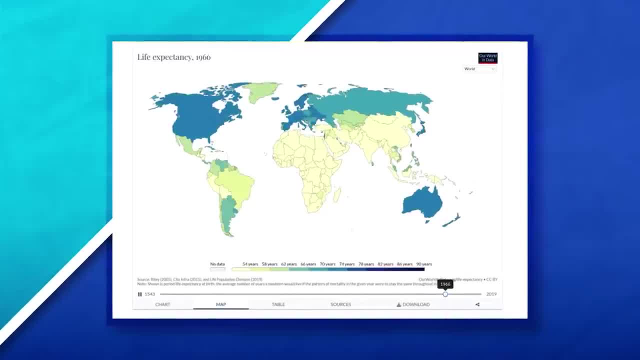 These changes in both the CBR and the CDR cause the NIR now to become more modern. As more people live in the cities, they no longer have the space or the economic need for larger families. Medical advancements in society lead to a higher life expectancy and decrease the infant. 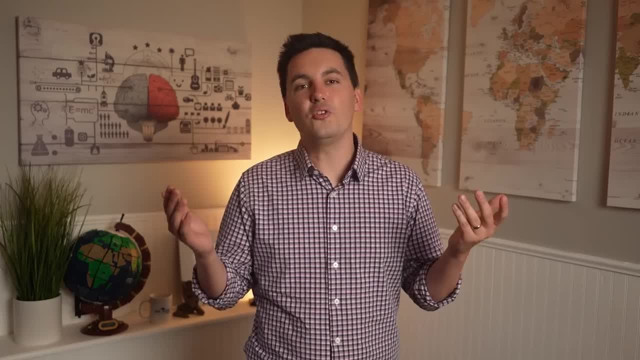 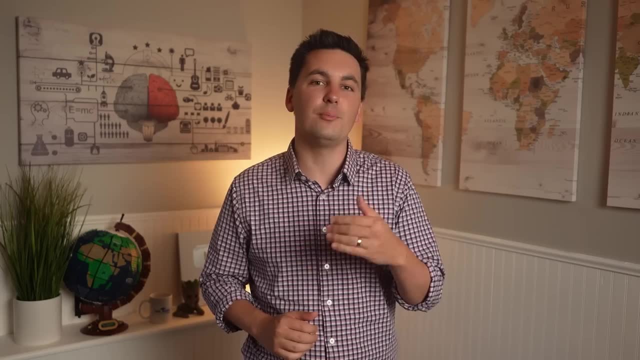 mortality rate. This leads to families having a fuller, more stable and more efficient life- less kids. We may also start to see cultural changes in society as well, such as how people view gender roles, which may often lead to women gaining more rights in society and being 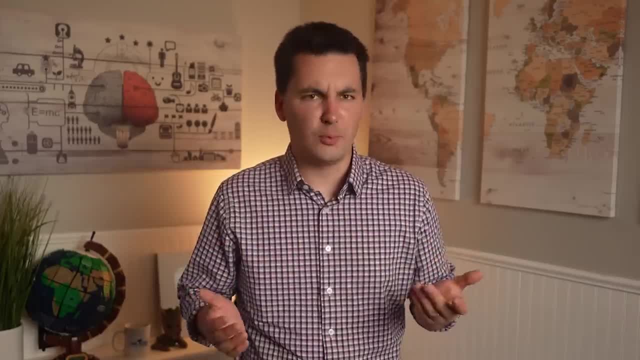 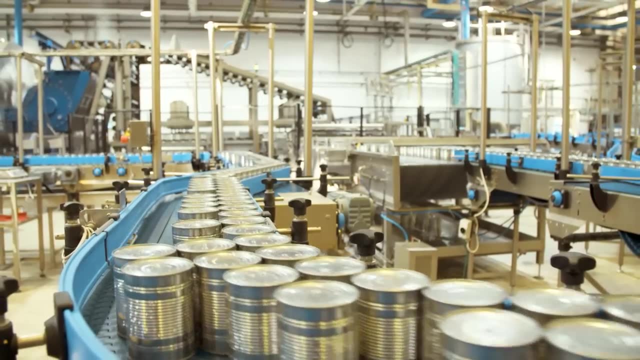 allowed to participate more in the economy. As society starts to develop, we start to see more and more jobs open up in the manufacturing sector, which would be part of the secondary sector of the economy. We also start to see more jobs starting to appear in the tertiary. 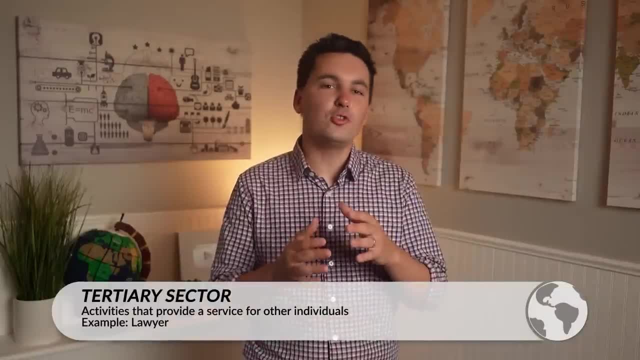 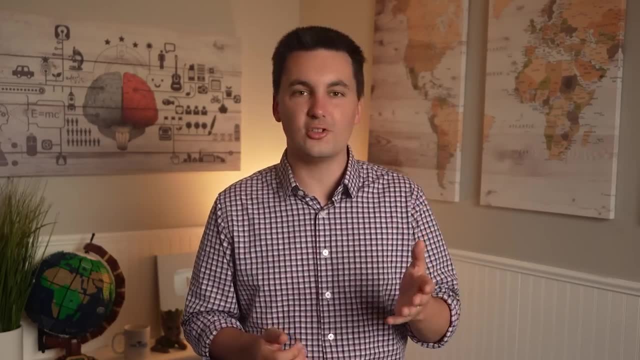 sector of the economy as well. These new economic opportunities also shift migration patterns as well. Traditionally, we see that less people emigrate from a country that has more jobs in the secondary and tertiary sector. As the economy advances, migrants will stay in their 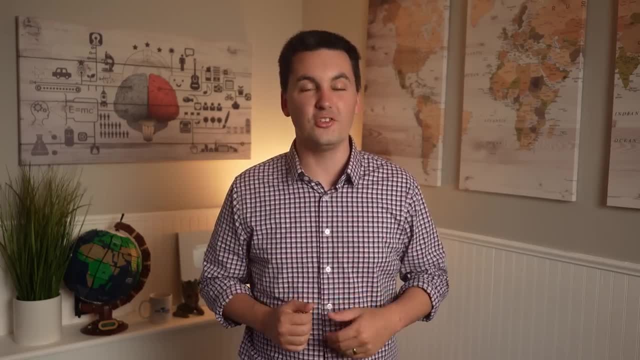 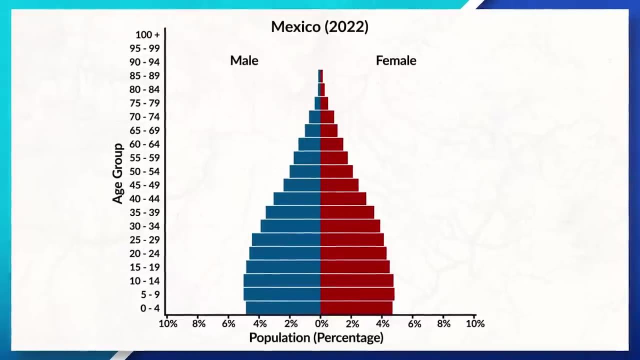 own country to be able to explore the economic opportunities that exist at home. Today we can look at Mexico as an example of a stage three country. Notice that when we're looking at Mexico's population pyramid, the middle of the pyramid is starting to fill out More. 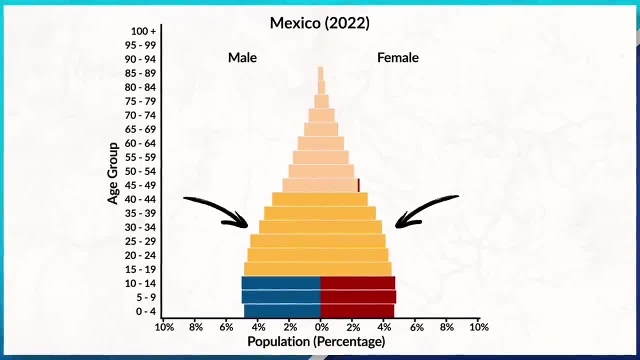 people in the country are now in their reproductive years and post-reproductive years. We can see that Mexico is still growing, but it's still growing. Mexico is still growing as a country, but not as fast as it would have been if it was. 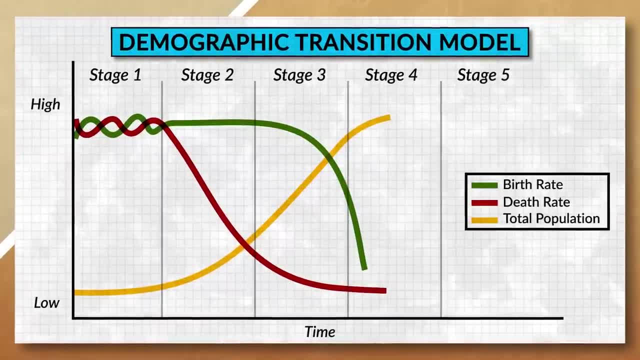 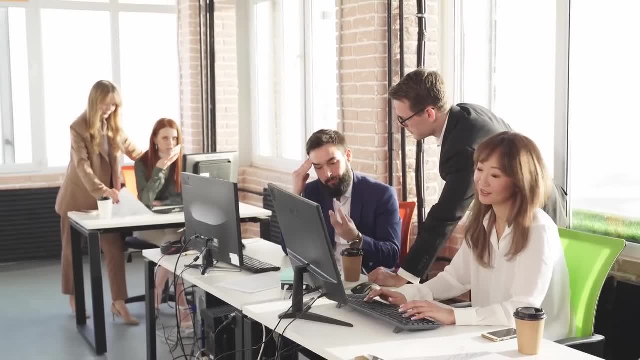 in stage two. Next is stage four, which is defined by a low CBR and low CDR and actually now a low to flat NIR. Here countries start to see more economic opportunities for all citizens, higher rates of education for women, more jobs in the tertiary sector of the economy. 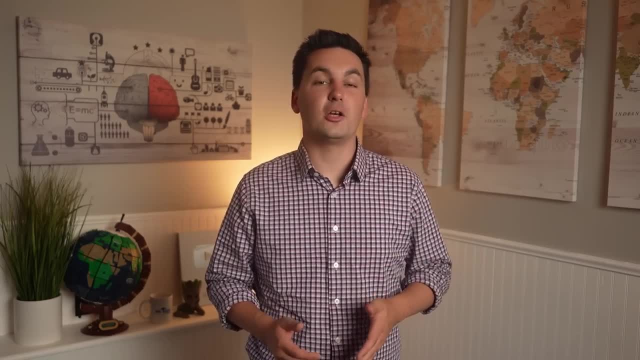 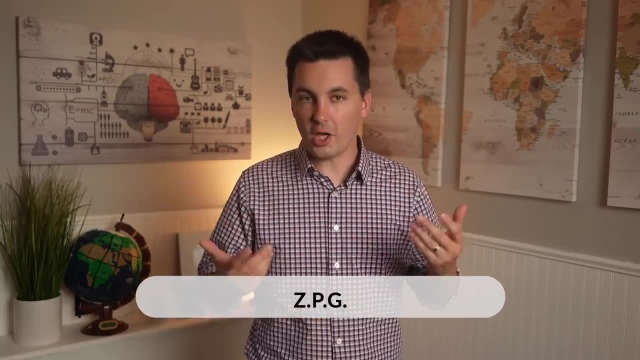 and more intra-regional migration. During this stage, countries may experience ZPG, which is zero population growth. This means that the country's CBR and CDR are essentially the same, causing the NIR to be zero. This demographic shift occurs for a variety of. 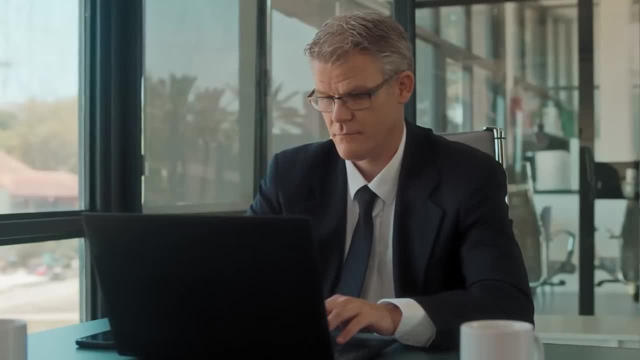 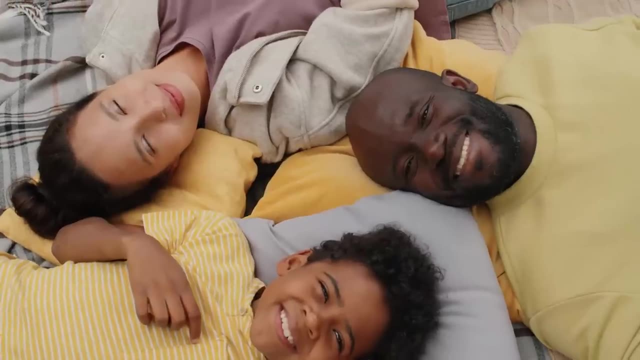 different reasons. We can see that, economically, more people are focused on their career and start to get married later in life, which causes them to have children later as well, which, of course, leads to smaller family sizes. As the economy grows, we will also see the 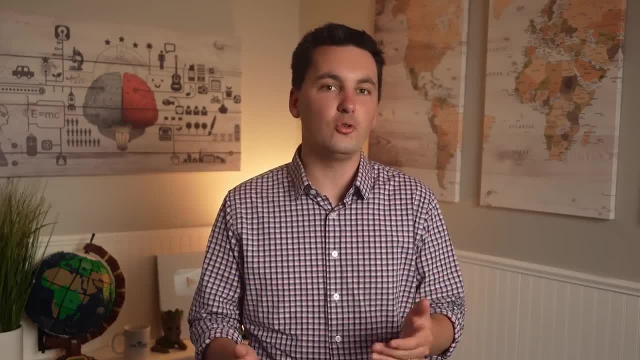 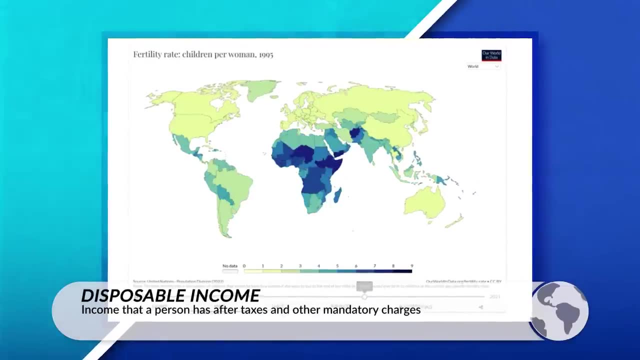 cost of living increase, which decreases the amount of disposable income that individuals have, which will further decrease the TFR of a society as people start to feel like they can no longer afford to live on their own. As a result, people will start to feel 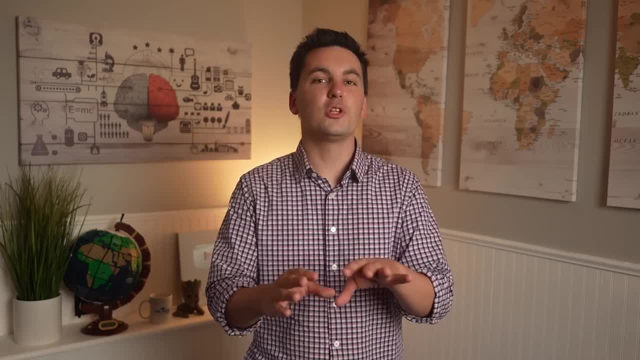 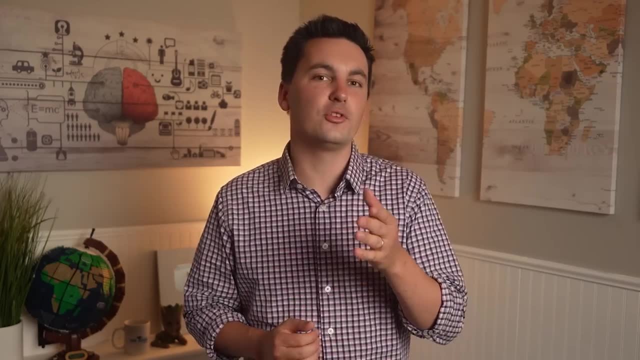 like they can afford to either start a family or support a larger family. Culturally, we start to see society offer more education and opportunities for women during this stage, which allow women to play a more active role in society and the economy. This shift also allows women to pursue their own careers and goals instead of being seen. 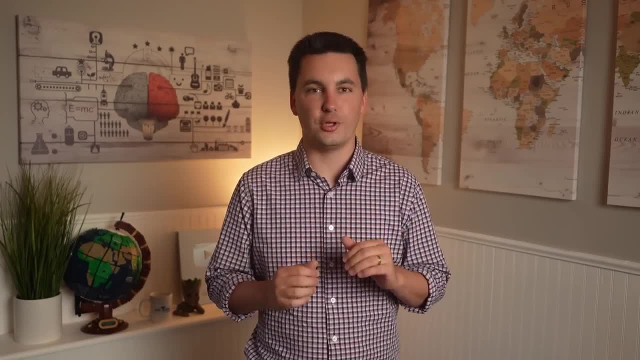 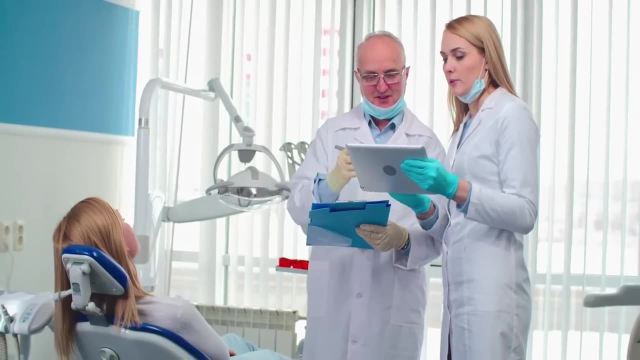 as childbearing. All these societal advancements help further decrease the society's CDR and IMR. As people continue to gain more access to wealth, they also gain access to better healthcare services and more nutritious food, which helps increase the average life expectancy and decrease the death rate. 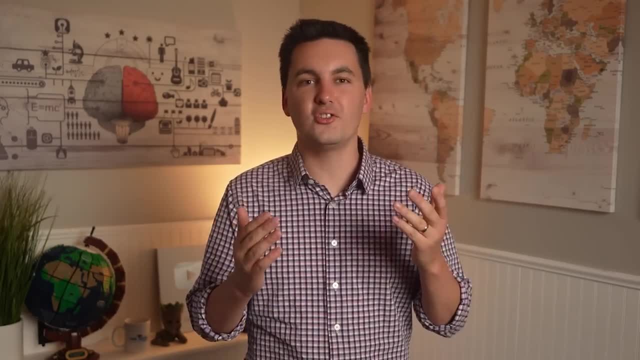 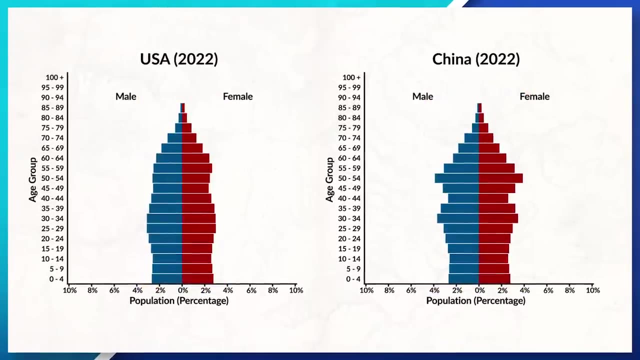 Today we can see that countries like the United States and China are good examples of a stage 4 country. If we look at their population pyramids, we can see that they form more of a box shape. Notice that the population is spread out between the different age cohorts. 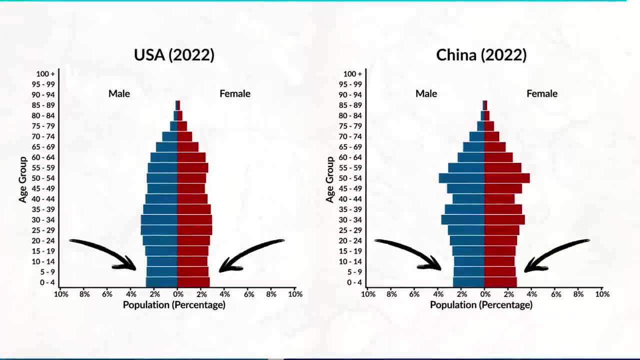 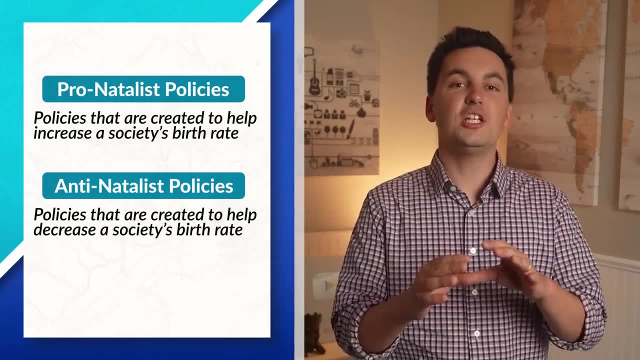 And while the countries are no longer seeing a large population boom, they are also not seeing a large decline. Now I do want to highlight that sometimes a country may move between stages due to political policies which can either promote people to have more children or deter people from having children. This is a very common situation in the United States. 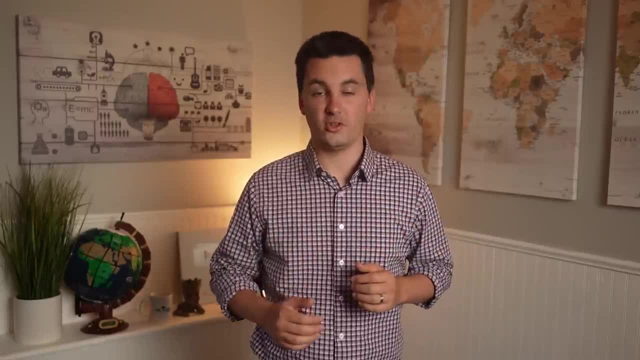 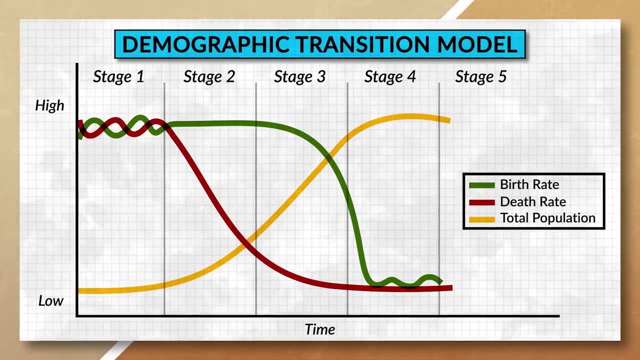 and I think it's important to keep that in mind. Government policies, such as the one-child policies, are what helped China transition into stage 4.. But we'll talk about those policies more in our Unit 2, Topic 7 video. Lastly, there is the speculative stage 5, which is defined by a negative NIR. Here. 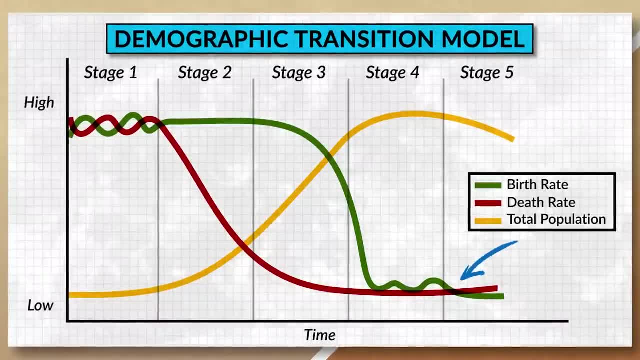 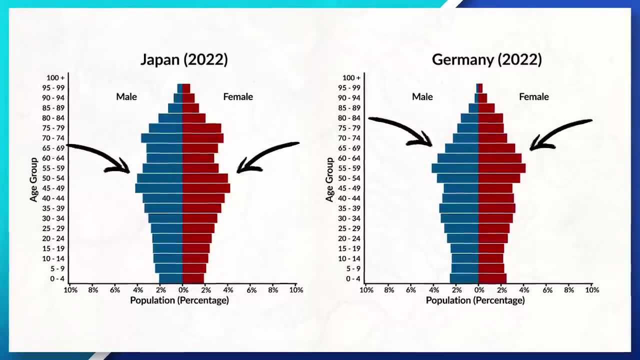 a country's birth rate goes below the CDR, causing the country's population to decrease. Countries that could be in stage 5 would be Japan or Germany. Notice how the majority of their population is located in the post-reproductive years on their population pyramid, Both of 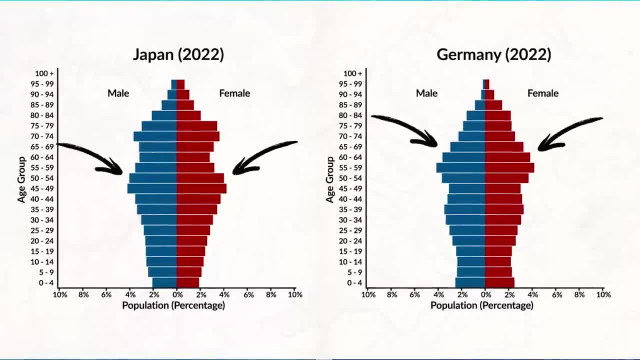 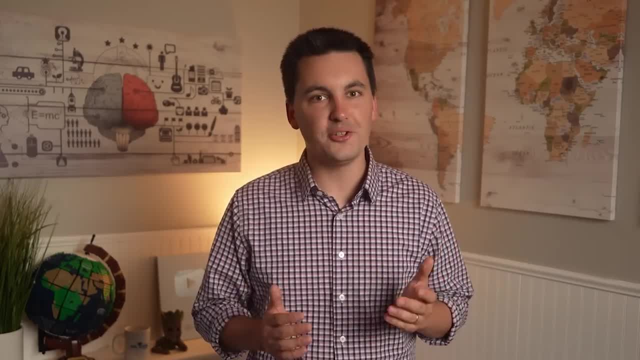 these countries have a negative NIR, Which means their overall population is decreasing. In order for a country to be growing, they have to have a TFR above 2.1.. This is known as the replacement rate. If their TFR is below, 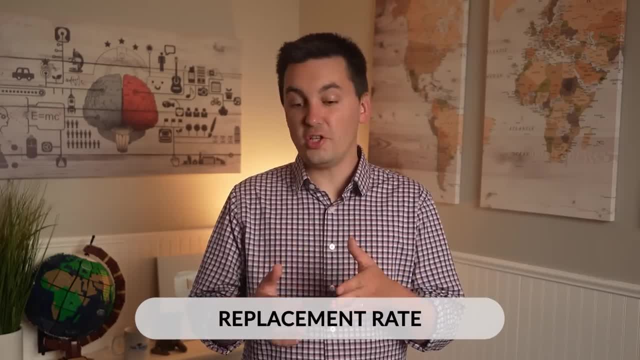 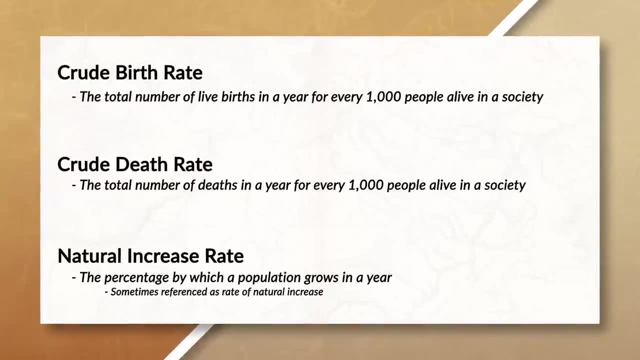 2.1,. the population will decrease over time. Remember, though, migration can change this, And when we're talking about the CBR, CDR and NIR, we are looking at births and deaths that take place in the country. These indicators do not factor in immigration or emigration. 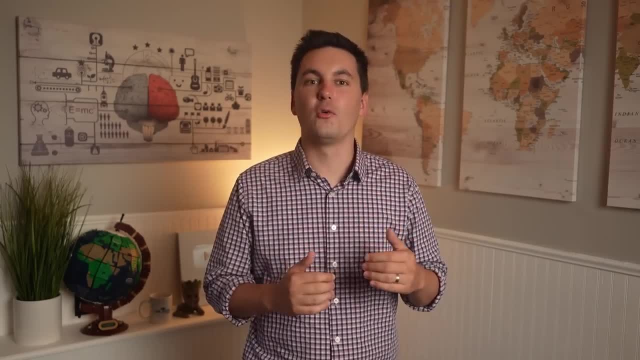 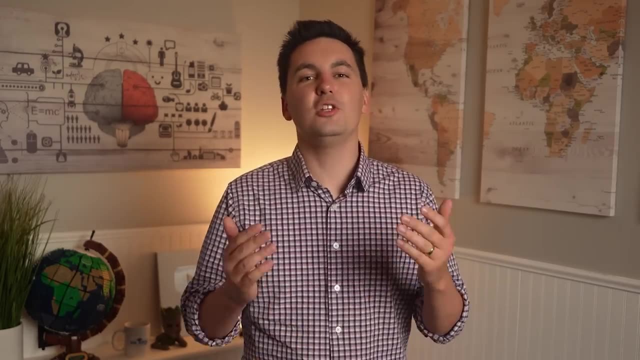 Okay, so that's the demographic transition model. Next we have to go over the epidemiologic transition model, But before we do, don't forget to hit that subscribe button. if you're finding value in this video And if you need some more help with your AP Human Geography studies, check out my ultimate review packet. 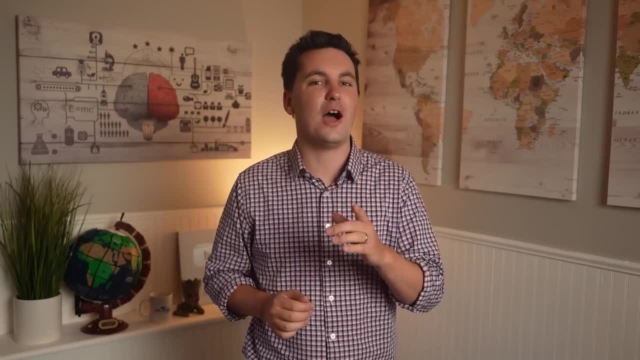 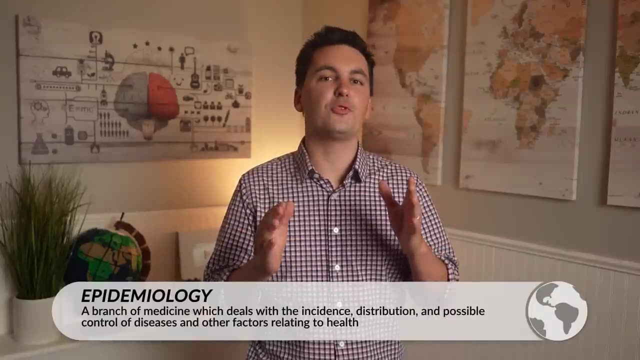 and Discord server. It's a great resource and it'll help you get an A in your class and a 5 on that national exam. Now the epidemiologic model goes along with the demographic transition model. There are a couple differences, but for the most part, we can use this model to better understand. 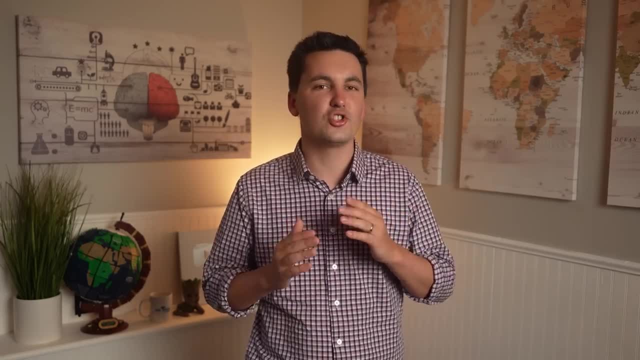 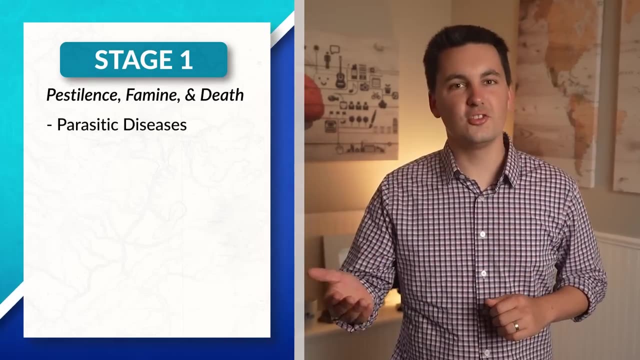 the different causes of death for each stage of the demographic transition model. Stage one is defined by pestilence, famine and death. Here people are going to die from a variety of different things: Parasitic diseases, infectious diseases, animal attacks. 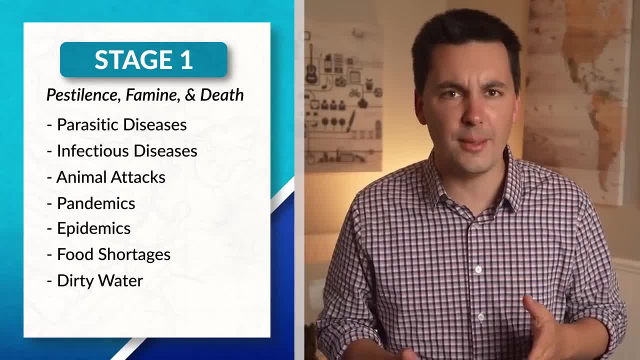 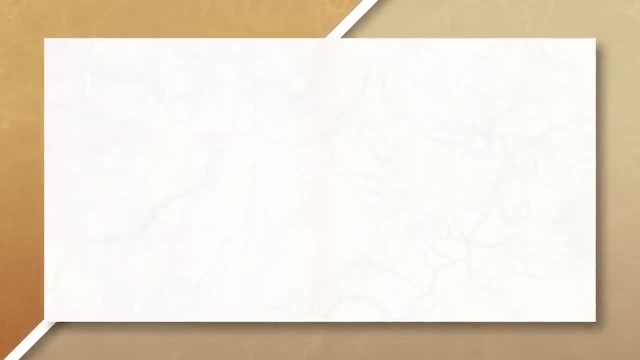 pandemics, epidemics, food shortages, dirty water, you name it. you can die to it. One of the most well-known killers in this stage was actually the bubonic plague. Now, I mentioned epidemics and pandemics, Remember, an epidemic is a disease that spreads through a region. 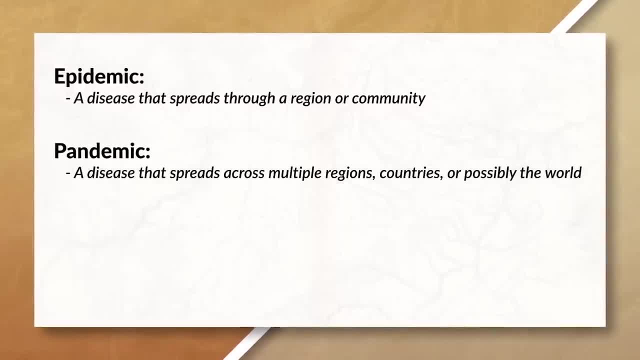 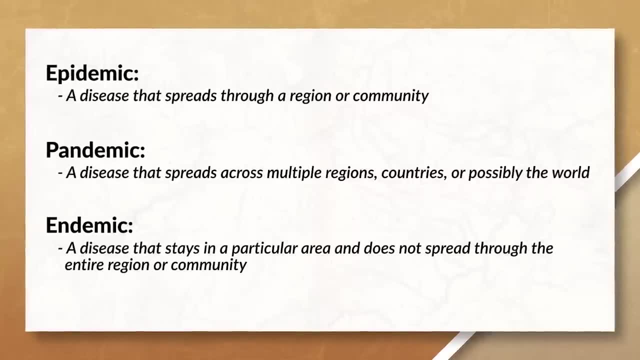 or community, And a pandemic is a disease that spreads across multiple regions, countries or possibly the world. Another term that you'll want to be familiar with is endemic, which is a disease that stays in a particular area and does not spread through an entire region. 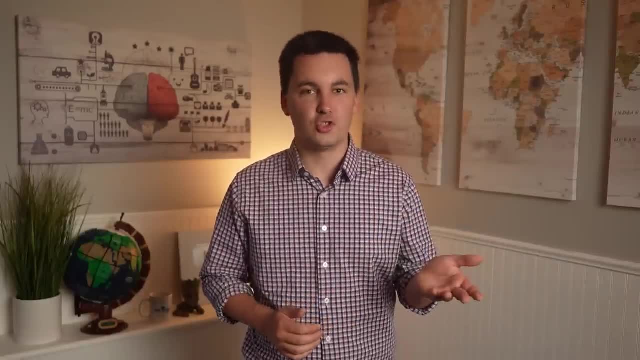 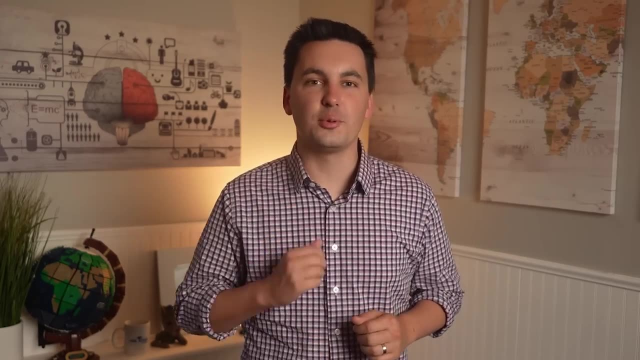 or community. Now, in countries transition from stage one to stage two, we start to see a decrease in the amount of deaths caused by major diseases. This is due to a variety of different factors, such as advancements in medicine, an increase in food supply and a higher standard of living. 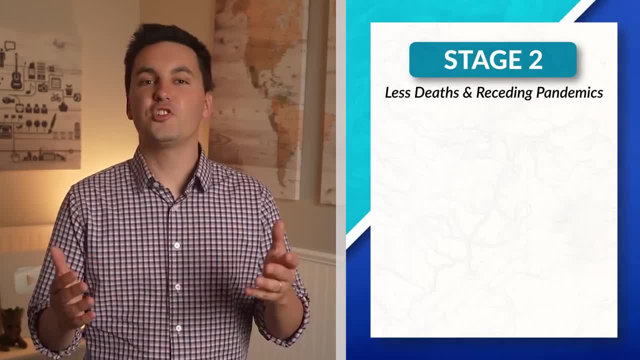 Stage two is defined by less deaths and receding pandemics. During stage two, society gains access to new technologies that improve health and well-being for people with disabilities. This is what we call a pandemic. The pandemic has not only improved the standard of living, but also helped increase the amount. 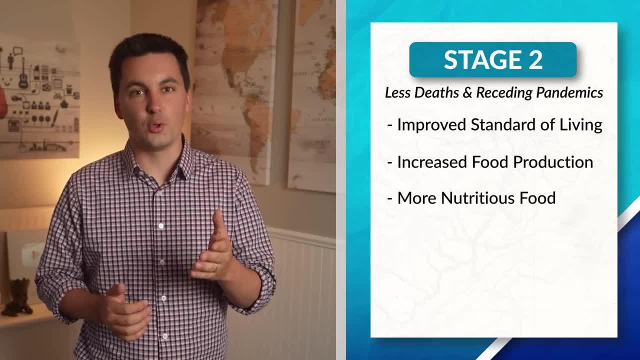 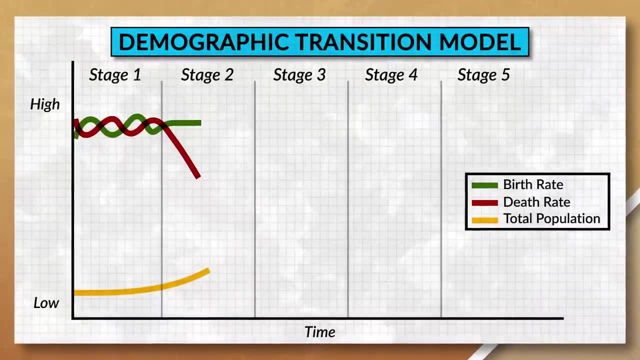 of food that is produced. Societies also start to eat more nutritious food and see improvements in sanitation as well. Remember, during stage two is when the industrial revolution and medical revolution occur. These events decrease a country's CDR but, like we talked about, 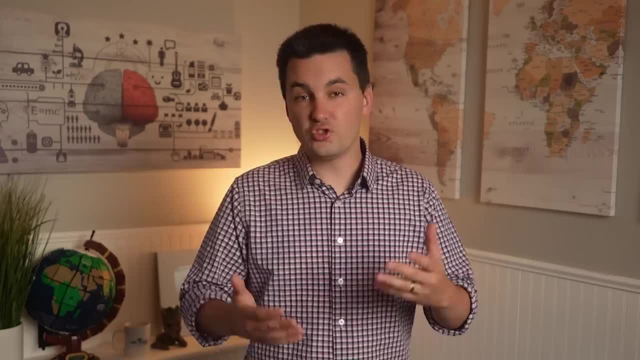 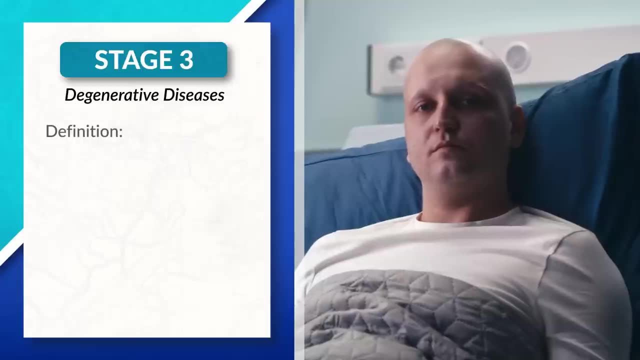 earlier in the video. do not decrease the CBR right away, which leads to societies to have a high NIR. As societies continue to advance, they eventually enter stage three, which is defined by degenerative diseases. Here people start to live longer and start to die from diseases which are 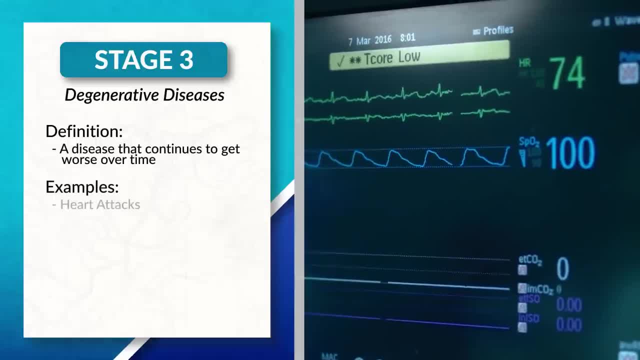 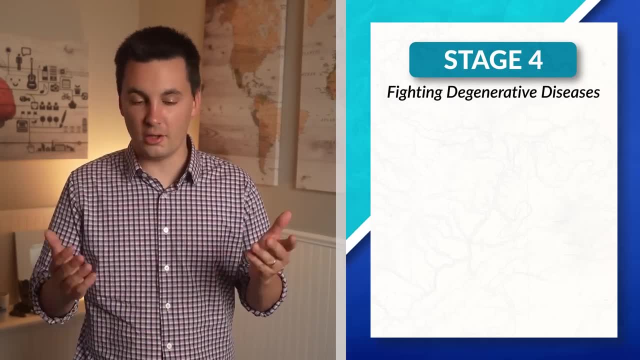 human-caused or caused by time, For example, heart attacks from eating unhealthy food or different types of cancer. Next is stage four, which is defined by fighting degenerative diseases and longer life expectancies. This is when medical advancements in society can delay degenerative diseases, which increases. 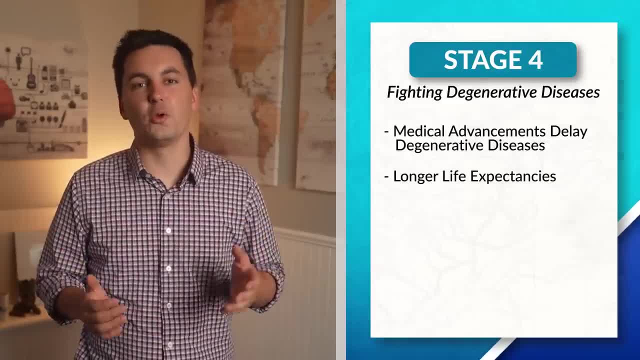 a society's life expectancy. During this stage, most individuals will continue to improve their diets with more nutritious food and make better health decisions. This is when people start to live longer and start to die from diseases which are human-caused or caused by time, For example, heart attacks from eating unhealthy food or different types of cancer. 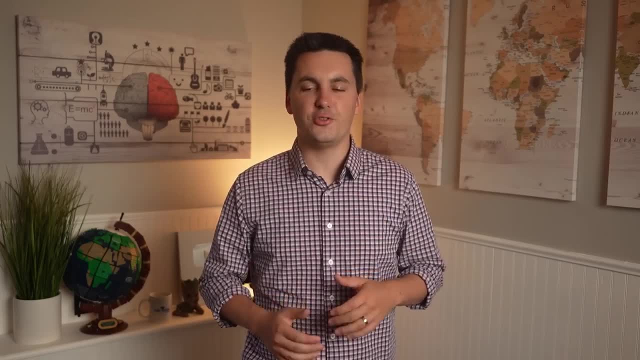 This is when people start to live longer and start to die from diseases which are human-caused or caused by time. This is when people start to live longer and start to live longer and start to die from diseases which are human-caused or caused by time. 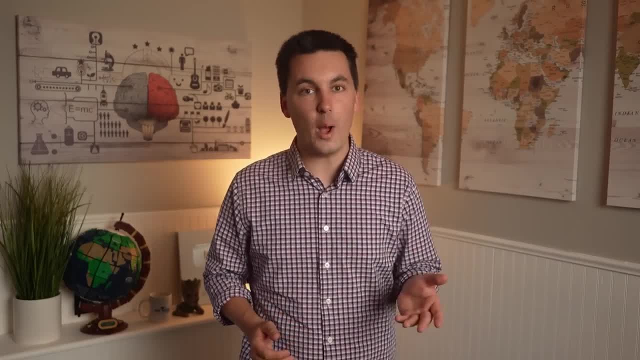 Like not choosing to use different drugs, But at the same time, we can see that these different advancements in society can also promote negative habits as well, such as living a more sedentary lifestyle or eating more junk food, which may lead to new health problems. 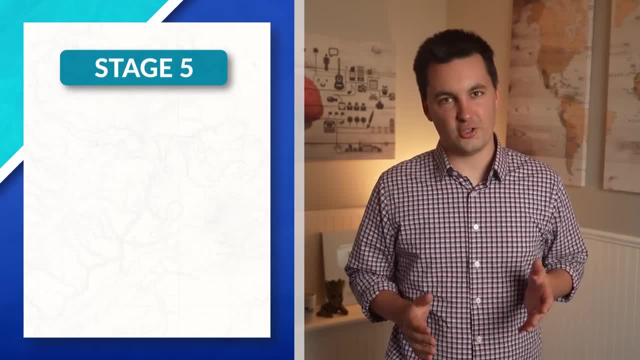 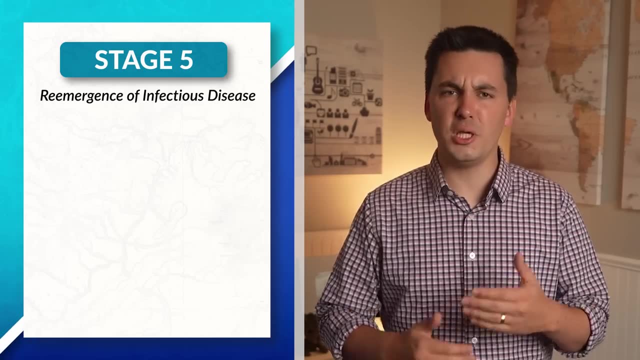 for individuals such as obesity or diabetes. The last stage is stage five, and it's defined by the reemergence of infectious diseases. During this stage, parasitic diseases and infectious diseases become more prevalent again. This can happen for a variety of different reasons. The first is the evolution of disease. 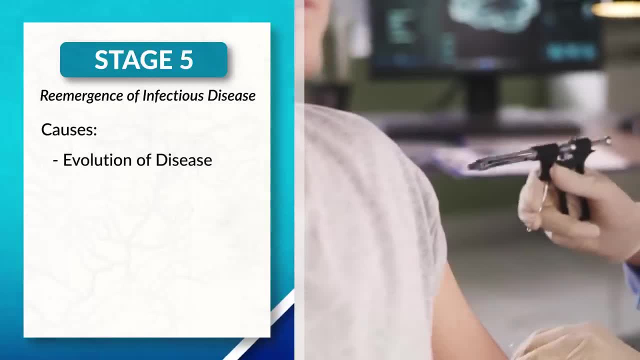 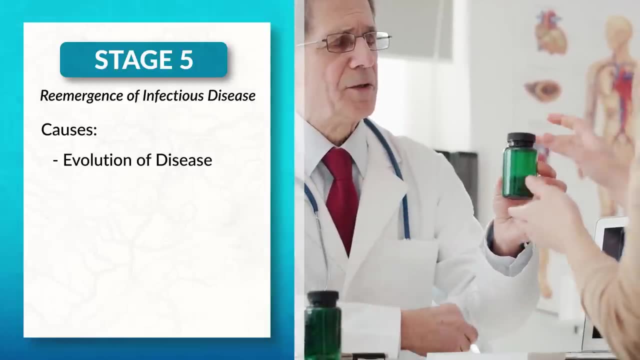 This is when a society sees different diseases mutate and develop a resistance to antibiotics. We can see that over time, as society continues to use antibiotics, we may see the development of superbugs, which are different strains of bacteria or viruses that are resistant to most antibiotics. 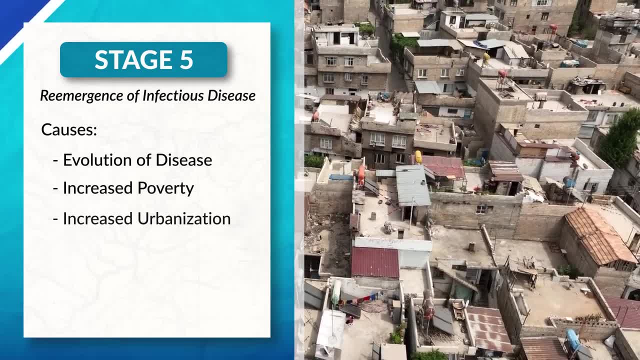 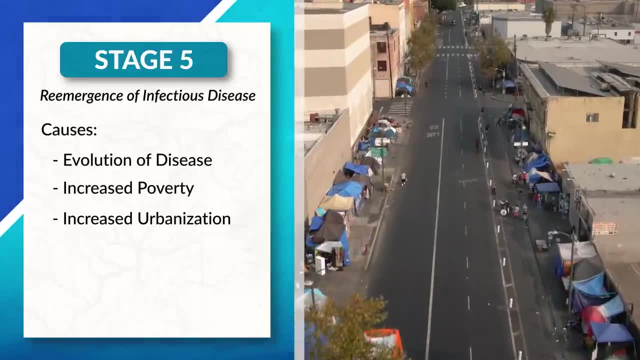 The next reason is an increased rate of poverty and urbanization. As cities become larger and more densely populated, it becomes easier for disease to spread throughout a city, And when people live in poverty, they are less likely to be able to afford different medication. 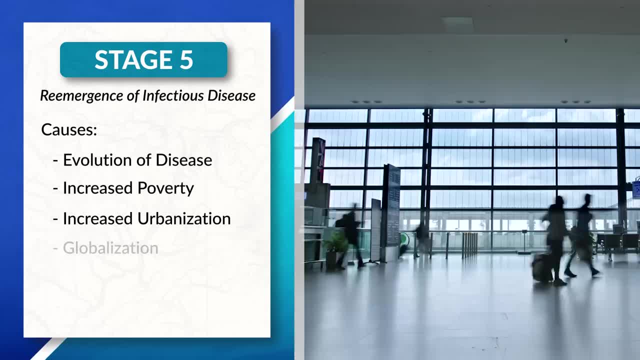 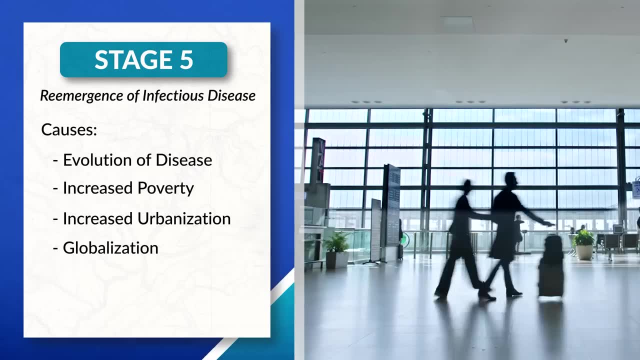 and healthcare services, which can lead to an increase in the CDR. Lastly, there is globalization. When people travel around the world, they gain experiences, share ideas, but also, at the same time, they share germs. This global travel and connectivity, 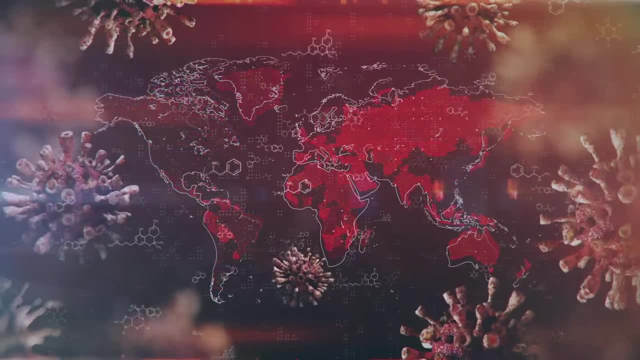 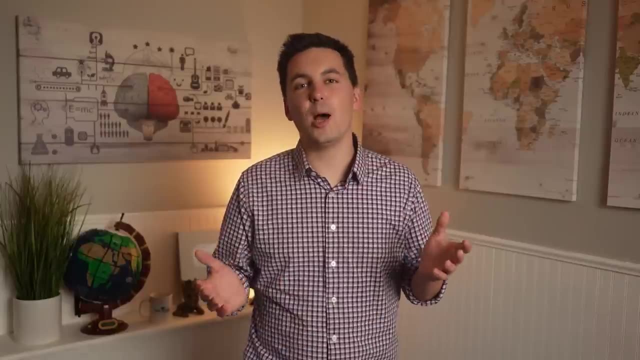 can lead to pandemics such as COVID-19.. We saw that cities that had large international airports and densely populated areas saw COVID-19 spread through their communities first. We also saw people who were in lower income brackets had higher rates of COVID, since they had less. 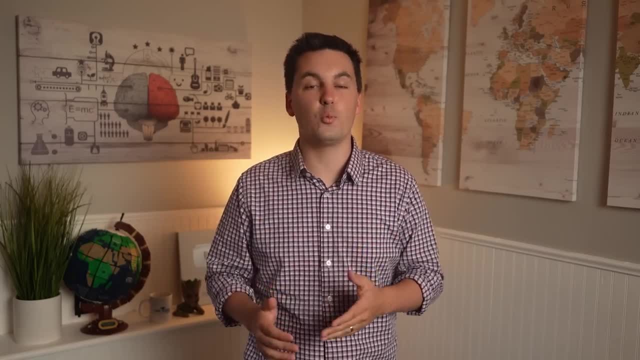 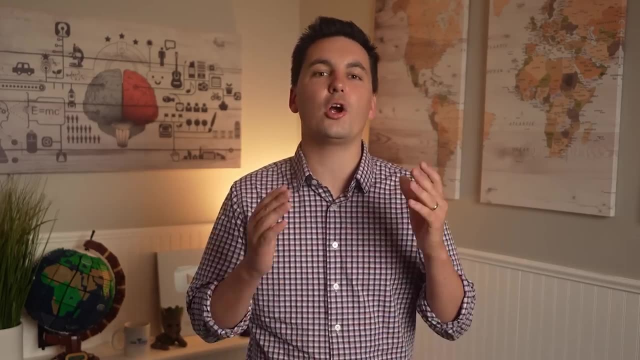 access to healthcare services and were more likely to be working in jobs where it was more likely to be exposed to the virus. Now, both the demographic transition model and epidemiologic transition model are important models for this class, so you'll want to make sure that you're familiar with both of. 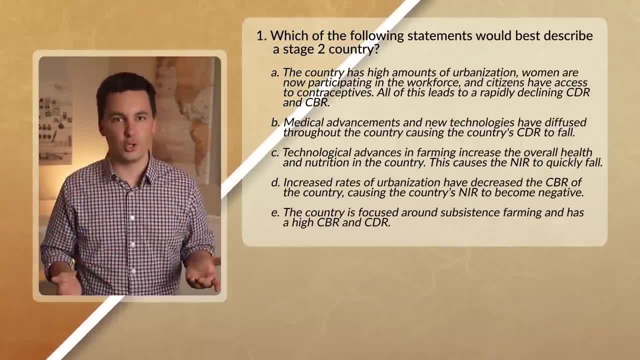 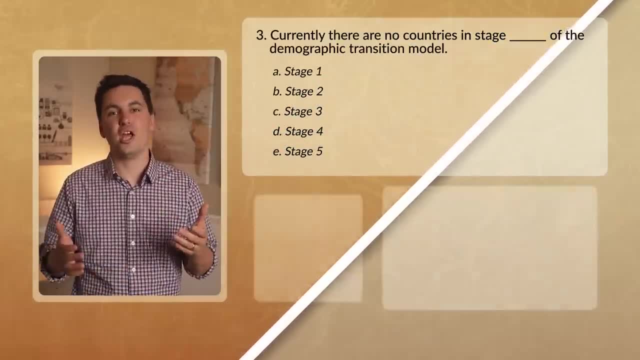 them. Alright, now you know the drill. Now comes the time to practice what we have learned. Answer the questions on the screen and, when you're done, head on down to the comments section below or the description of this video to check your answers And, if you feel like, 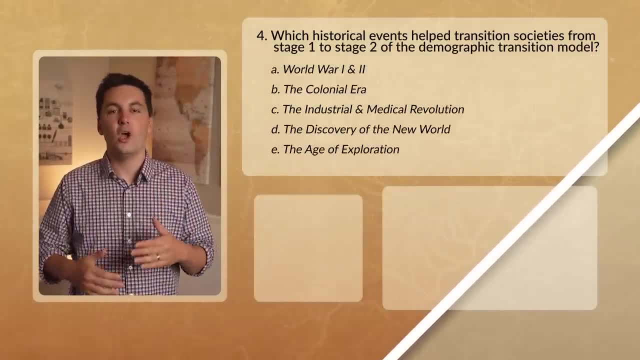 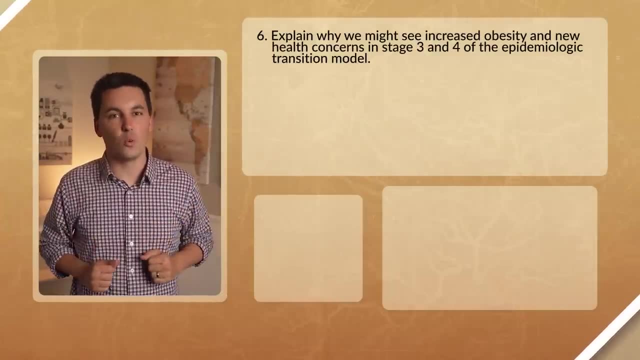 you need some more practice with these models. head over to my Ultimate Recipes channel to read my Ultimate Review Packet for more help with not only just these models, but everything else AP- Human Geography related. As always, thank you so much for watching. I'm Mr Synn and I will see you. geographers. next time online.